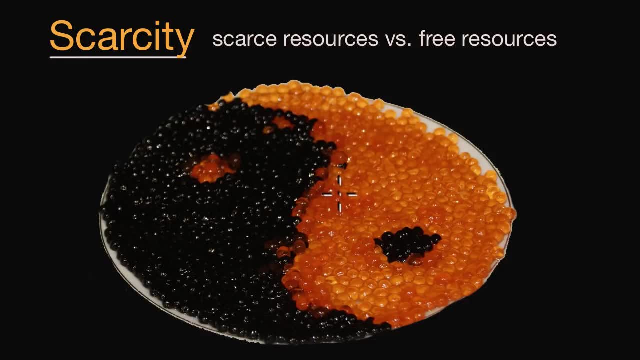 as much caviar as I want- and there's still as much as you want- and that everyone gets as much caviar as they like. Well, that's clearly not the case. Caviar is a scarce resource. In fact, it is a quite scarce resource. 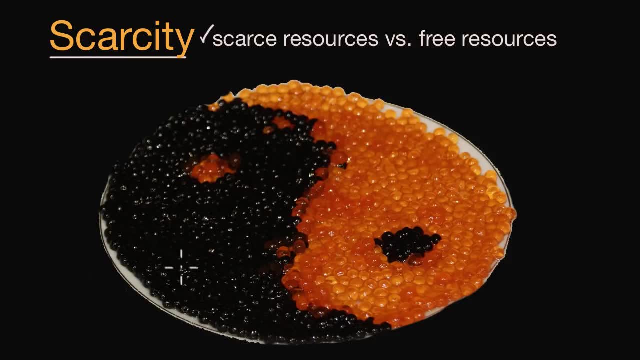 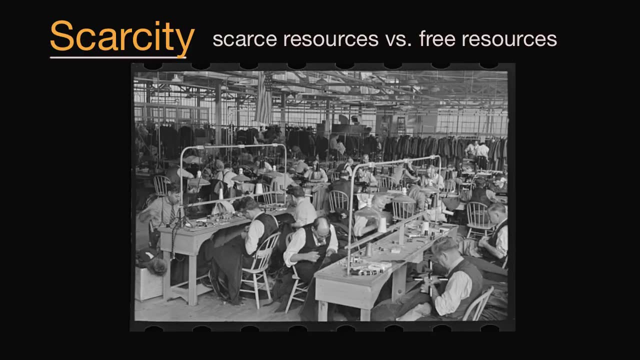 and because of that, if you want it, you have to give up a good bit to get it. This is a picture of some people working in a factory, and the resource that jumps out here is that of labor, And labor's interesting because it's not as tangible. 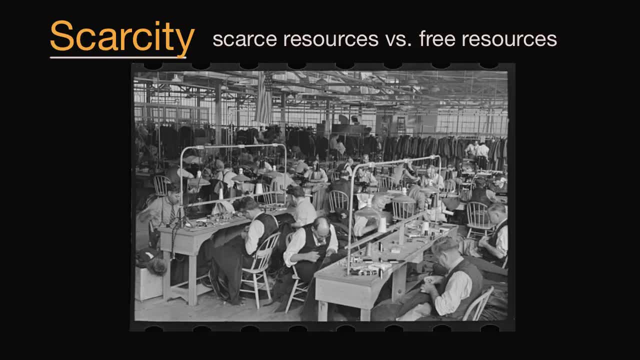 as something like caviar, but it is a resource And one could even argue that the caviar on your plate, some of its scarcity, comes from the labor involved of getting it to your plate. But here these are. clearly it looks like these are gentlemen. 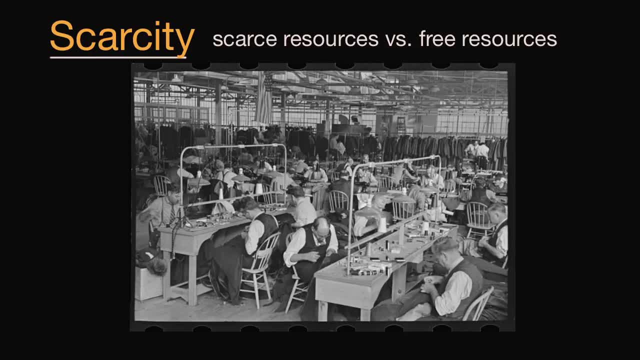 who are putting together some type of fabric, And so would you consider labor. would you consider that a scarce resource or a free resource? Well, it would be a free resource if people were willing to just do as much work for other people actually willing to do an infinite amount. 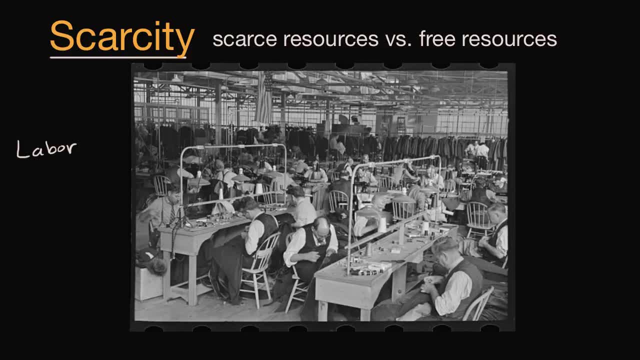 of work for other people, which isn't even humanly possible. And even if it was humanly possible, people aren't willing to do that. They want something in return, And so, once again, it is a scarce resource. There's many resources that are pictured right here. 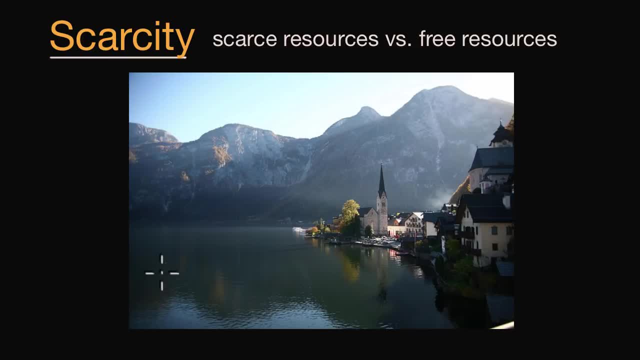 You have this beautiful town next to this alpine lake, And so some clear, scarce resources are here. Many people would love to have a view like you would get from this house or hotel right over here, but not everyone would like to have a view like this. 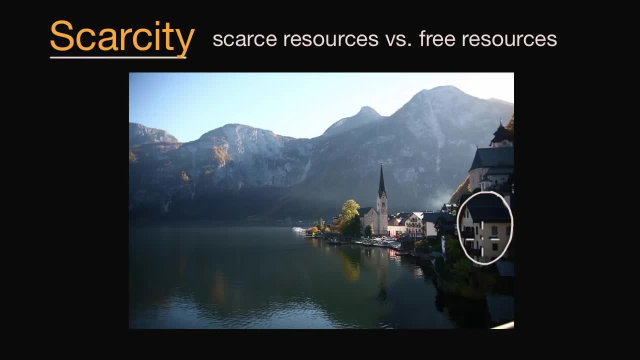 Many people would love to live there because of the view, but not everyone can live there, So that is a scarce resource. The water here is an interesting one. I could imagine in earlier times if before there was a town here, if there was just a primitive village. 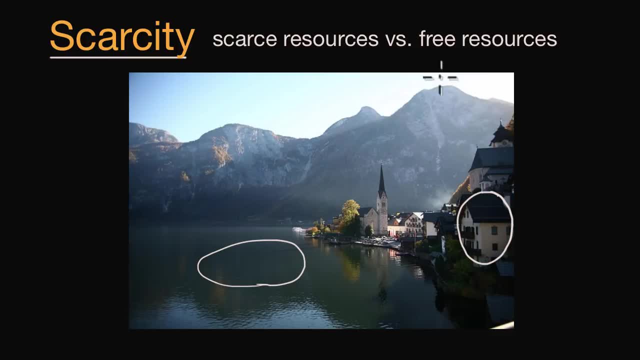 living next to this fresh water, they would probably view it as a free resource. If someone was thirsty, they would just go up to the lake and they would just drink from the lake. They would not have to give up anything to drink from that.